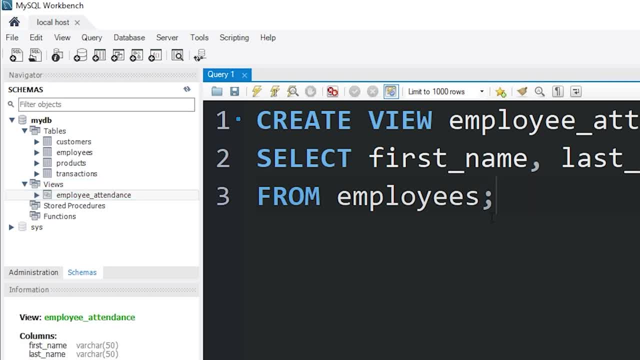 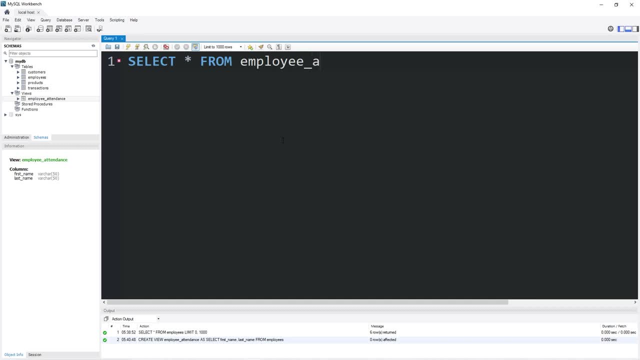 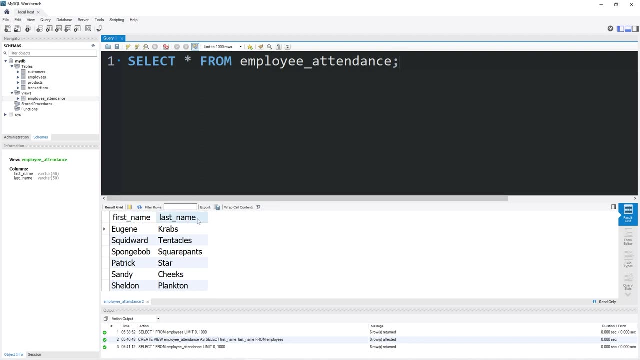 category. we have a new view- employee attendance. I'm going to select all from that view name, employee attendance- And let's see what we got. Yeah, here's our attendance sheet. We have the first and last name columns from the employees table. This view is going to be the first and last. 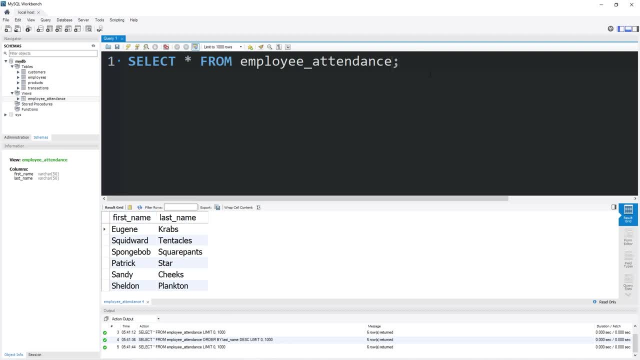 name. Each of the views in the view can be interacted with as if it were a real table. I will add order by last name ascending. You can use keywords and operators that we've learned about in previous lessons. on a view To drop a view, you would type: drop view. the name of the view: employee attendance. 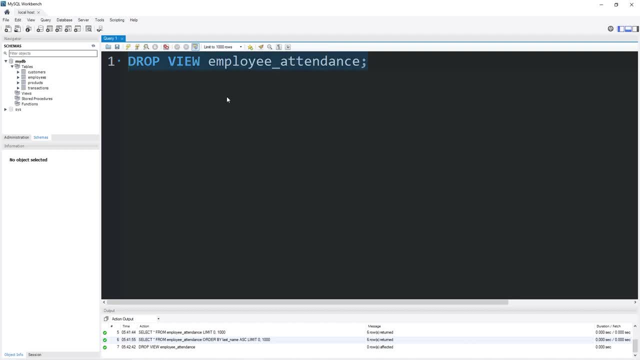 And it's gone All right. here's another example. So views, they're always up to date, right? I'm going to. they're always up to date, right? Let's create a view of customer emails. Select all from customers. 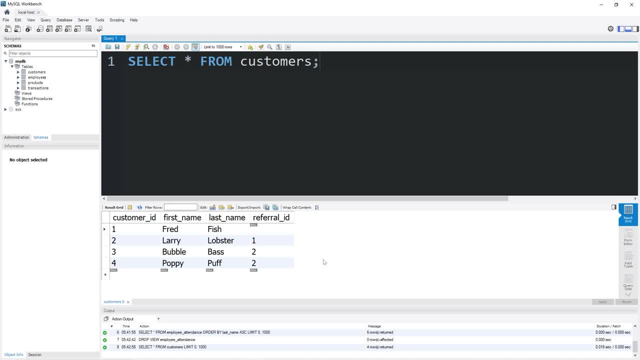 Let's take a look to see what we have so far. I'm going to add one more column, A column of customer emails. Alter table customers, Add column email. Data type will be varchar. I think varchar 50 should be enough space. And there's our new column. Let's update these rows. 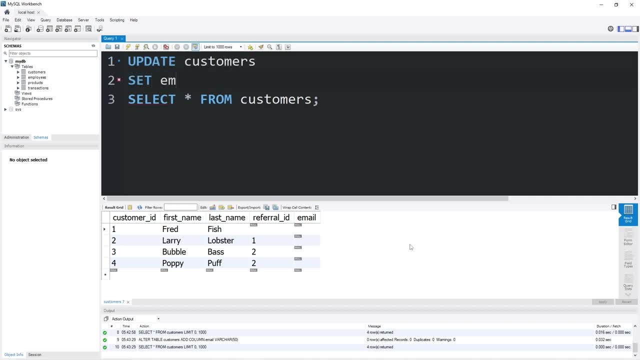 Update customers set email equal to. The first email will be for fred fish, f fish at gmailcom. Then we'll need a where clause Where customer id equals 1.. That's our first email Customer id. 2 will be l lobster at gmailcom. Three is b bass at gmailcom. Four will be p puff at gmailcom. 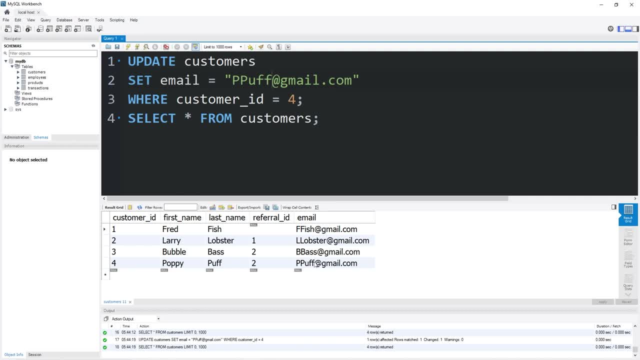 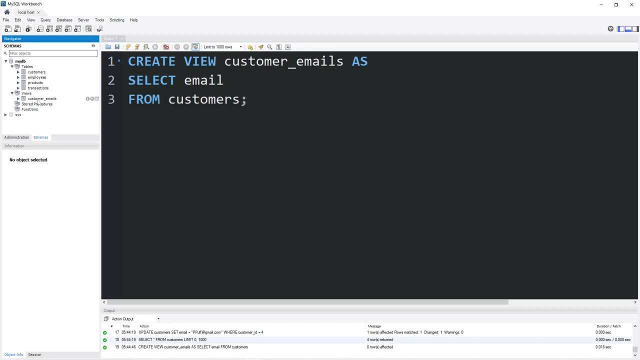 Everybody really likes gmail, I guess Let's create a view from these customer emails. Create view customer emails as. what are we selecting? Let's select the email column from our customers table. Let's refresh our schemas window. Yeah, we have a customer emails view.